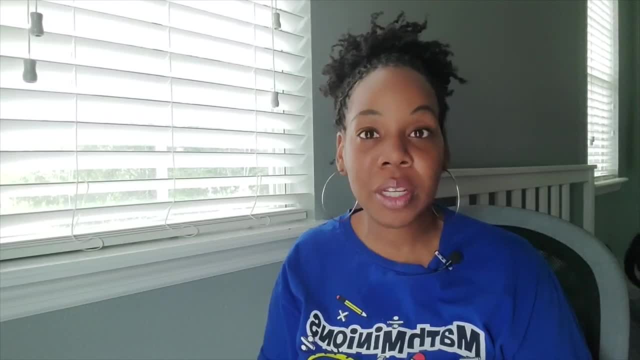 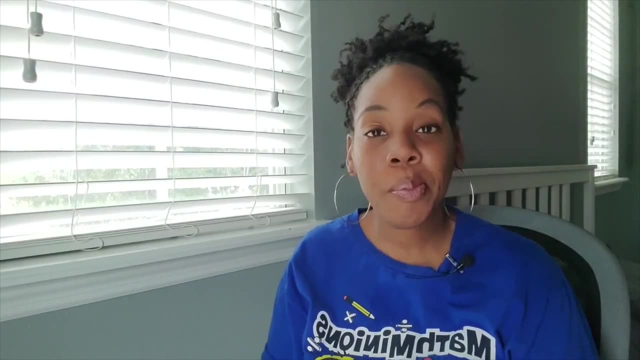 you can create a student data tracker for your students using Google Slides so that they can track the progress that they're making with their assessments over the school year, And if you're a parent, you can definitely use this resource too. Maybe your child's teacher is not tracking their 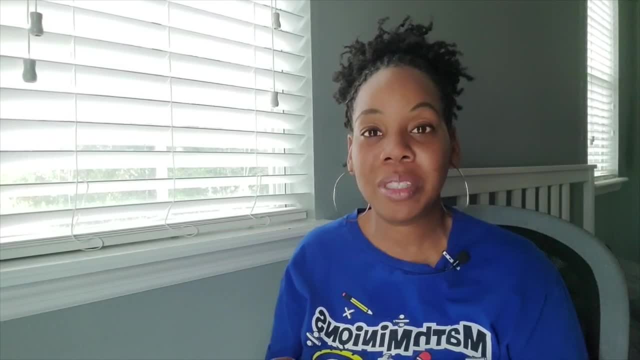 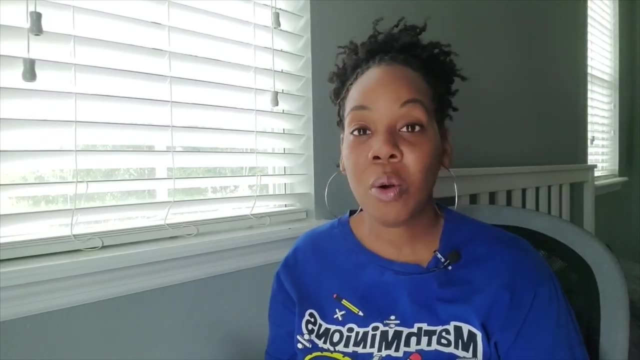 assessments over the year or not sending it home, but they're sending home those test scores. Maybe you want to track how they're doing on their assessments, whether it's a unit test, a chapter test, a quiz, a quarterly or some type of district test. So you definitely can modify this data. 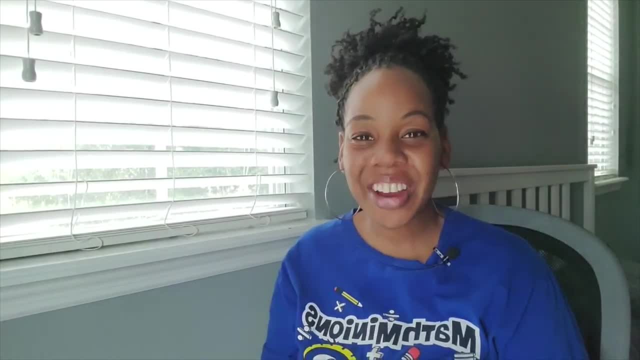 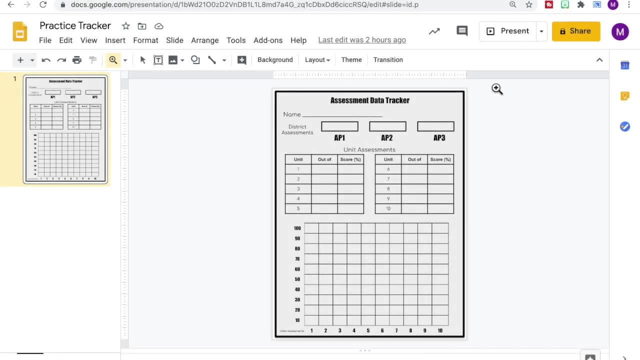 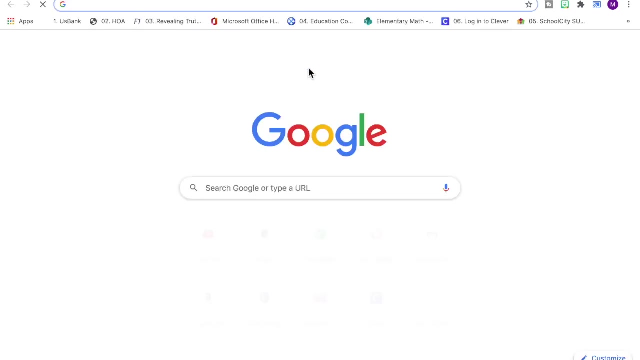 tracker to meet the needs of your child. Let's get started. In today's video tutorial, I'm going to show you how to make a student assessment data tracker, and we're going to be using Google Slides. I'm going to open up a new tab and, within Chrome, I'm going to go over here to my menu of Google Options. 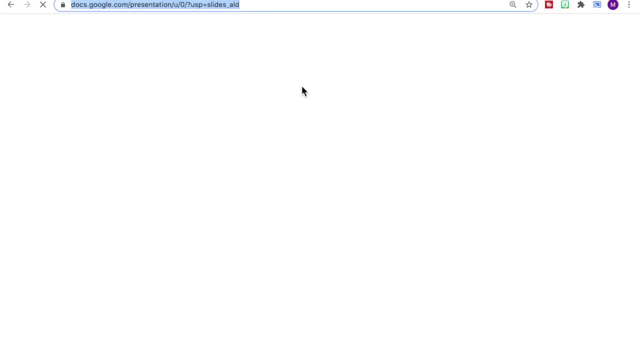 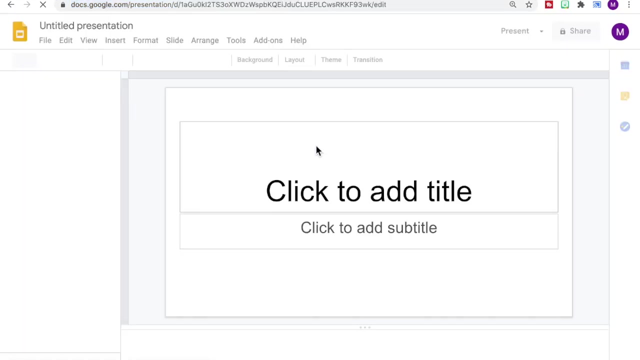 And I'm going to go to Google Slides and then click on a blank presentation to start start a new presentation. so I'm going to exit out of the themes that pops up automatically and go to file and then go down to page setup so I can adjust the. 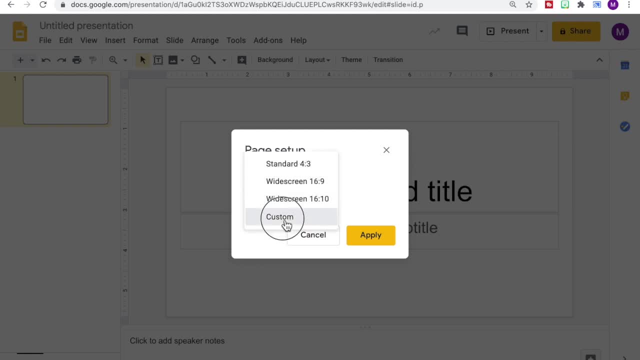 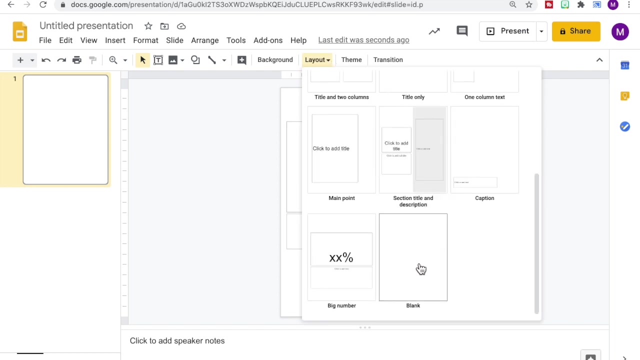 settings. I'm going to click on this drop down menu and then hit custom and change my dimensions to eight and a half inches by 11 inches, and then hit apply, and then I'm going to go over to layout and scroll down until I see the blank screen. 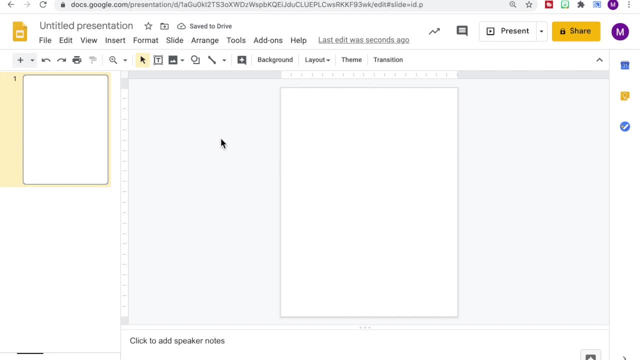 so we have our basic page, our canvas. now for our tracker. I'm going to start by adding in a text box. so up here in our ribbon, the T in the box is for text box, so I'm going to make one here. I'm going to start with the title, I'm just going 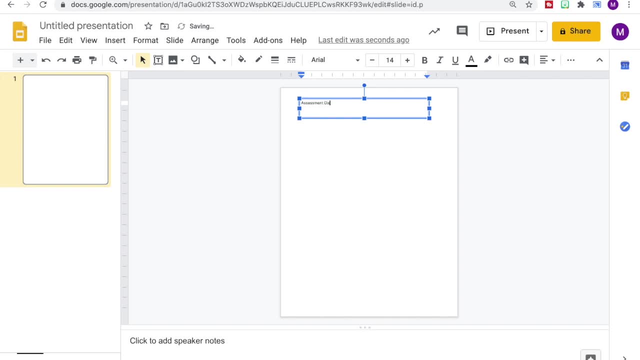 to put assessment data tracker. let's highlight that so we can change the font and the size of the font. let's go with impact and then increase the size. bring in our text box and then I'm going to center the text and then move it towards the middle of the page. 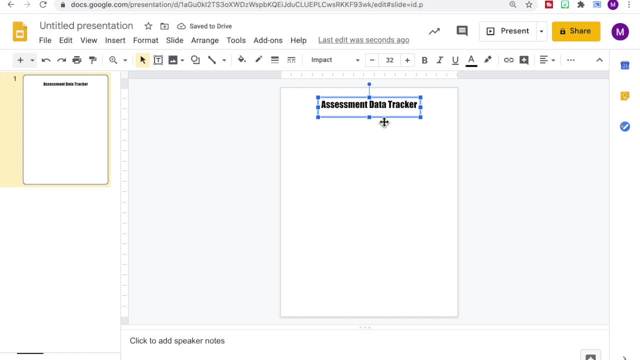 it's very similar to working in PowerPoint and canva, so there's our title. I'm going to click on this text box and hit command D on my keyboard so I can duplicate it, and then I'm going to change this so that I can have a spot for them to write their name. 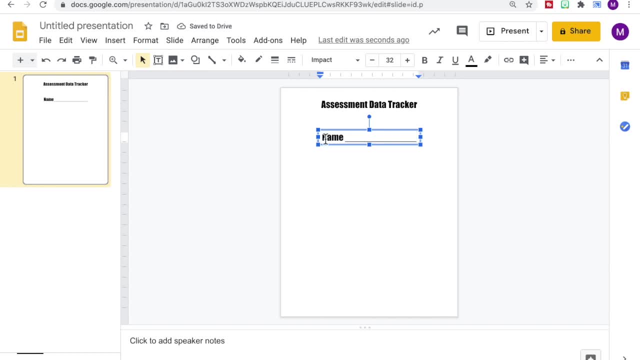 and then I'm going to change the font to a lighter font and then extend this text box so it all fits, and then I'll probably decrease the size of the font or of the name. so let's move that under. actually let's move it to the top and we'll move our title down. 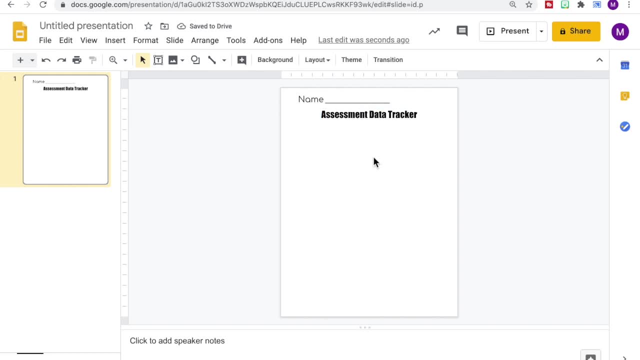 so, with our assessment, that data tracker, this is really a printable, a resource that you will modify and adjust to meet the needs of the assessments your students will be taking, for however long you want to track it. so you might track it for nine weeks, maybe a semester, or 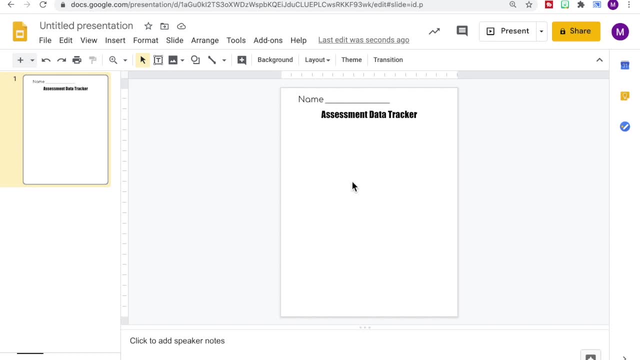 maybe the entire year, and there's different things you can put on here. you can put quizzes, weekly assessments, quarterly assessment, chapter test, whatever you want your students to track. so I'm going to track two different things. on this example, I'm going to track if a students take like a large 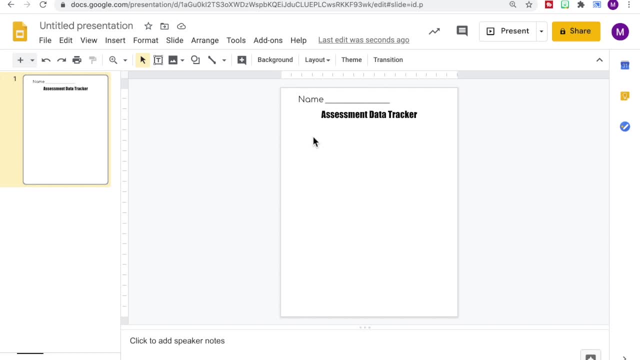 district or county assessment, and maybe they do it three or four times in the year. I'm going to add a shape. I'm going to add a square or rectangle for the students to write in their scores for each of those assessments. let's move this over here, and then I'm going to do: 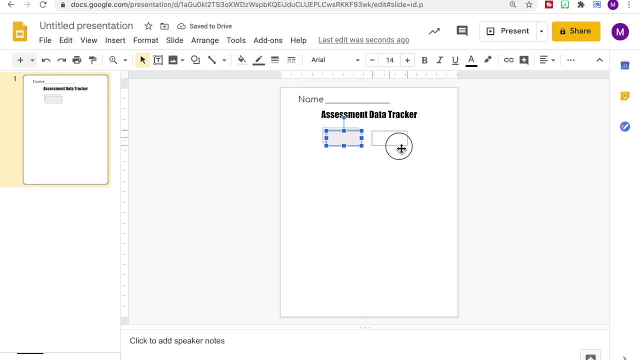 command D to duplicate it. I want to have three spots and then duplicate it again. and on Google slides you can just like hit or touch some of the text boxes and it will highlight the entire thing. in PowerPoint it's different. you have to highlight all of the text box in order to select it. so that is one of the 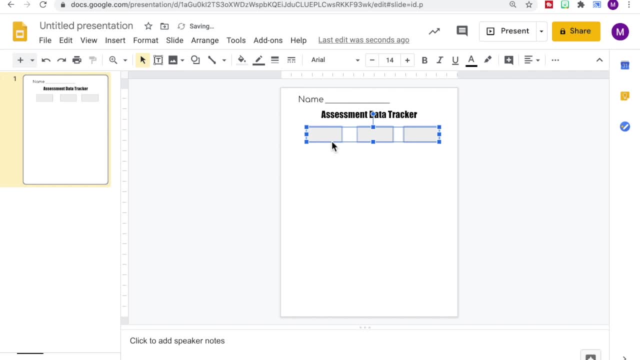 benefits of using Google slides when I move it over slightly, because I am going to put a border on the edge edges, so I want it to have space, and then let's make sure this is in the middle of the outside boxes. so now I'm going to add a text box. 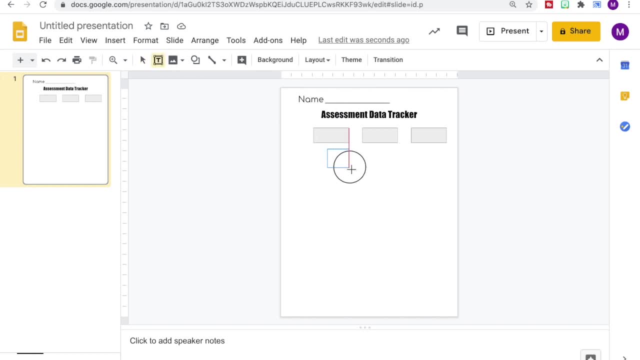 under each rectangle to write: I'm going to type in AP for assessment period and then the number one, so AP one. let's use that impact font again and then increase the size, and center it, and I'm going to put that right under that first box and then duplicate it. 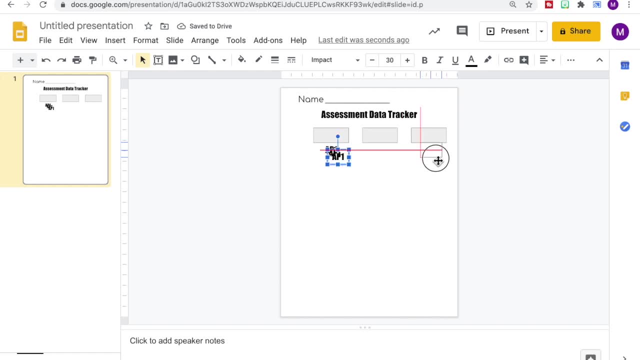 twice for the other two rectangles, and then we're going to change this to the number two and then the number three and, of course, if you have more or less make those adjustments on yours, and then I'm going to duplicate this one more time so we can label this right. 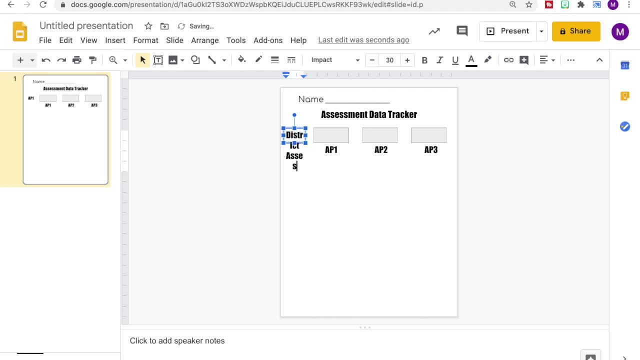 district assessments. ok, so that one is done. so next, what I'm going to do is add in a area, or two areas, for students to write their scores out for each of the assessments that they take their class or at their school. so let's just say that there are 10 units for the 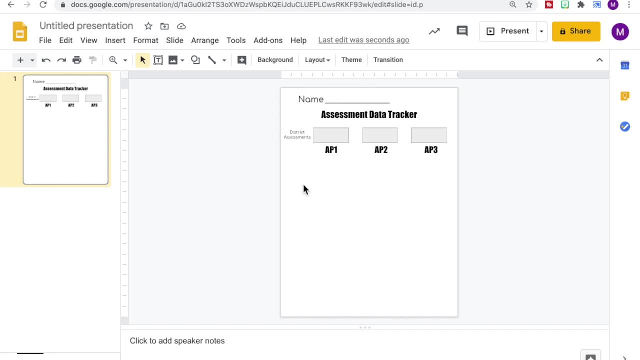 entire year, 10 math units or 10 chapters. so we're gonna have 10 places for them to write down their percent and they're the number that they have correct. so I'm going to go up to insert and then go to table and just hover here and it shows. 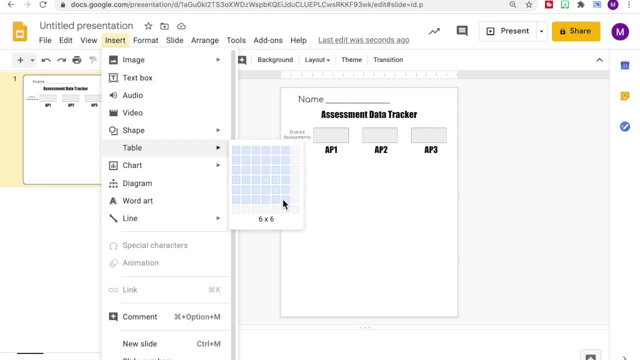 you the different dimensions you can use to create your table and I want to have five spots. so we're gonna do half on this chart and then make another half for unit six through ten. so I'm gonna so because I need five on this table. I'm 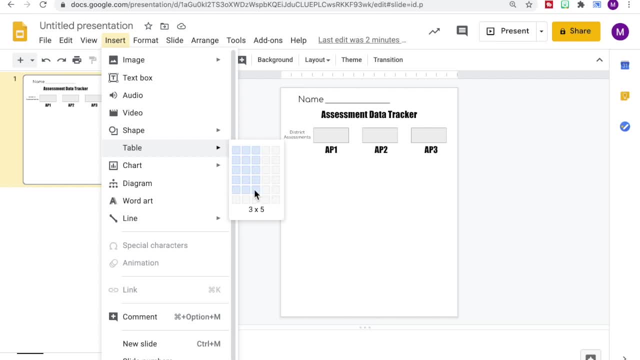 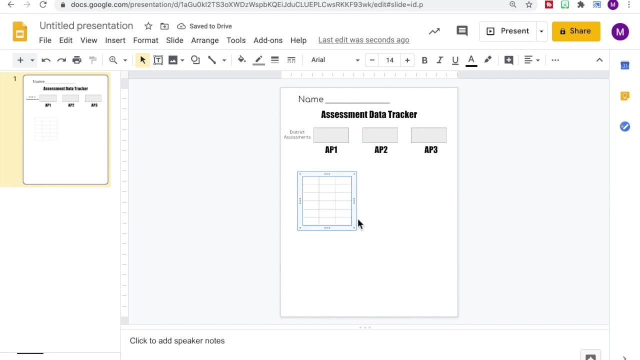 gonna add a six row so I can put labels. so let's do three columns of six, okay, and then let's bring it in and push it up here to darken the outline or the lines on the table. you're gonna select that table and then come up here to our 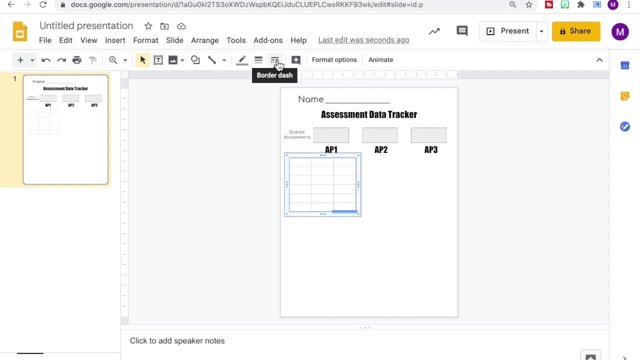 toolbar and we're going to select where it says border weight and make it three and then border color: we're gonna choose black. make sure you highlight it first and then do that. so I'm gonna go back and make the border color black and the border weight three. I'm gonna bring it. 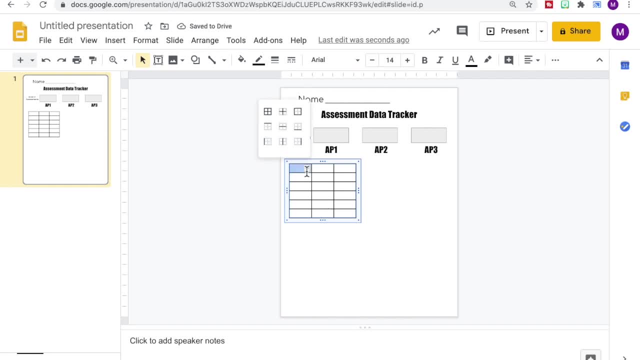 down some and inside I'm gonna highlight all of the cells and make sure they are centered and I want that top section to be bold, okay, and I want all of them to have this font. so in the first cell we're gonna put the units and we're going to put the out of score And then we're gonna put the score as a percentarte. 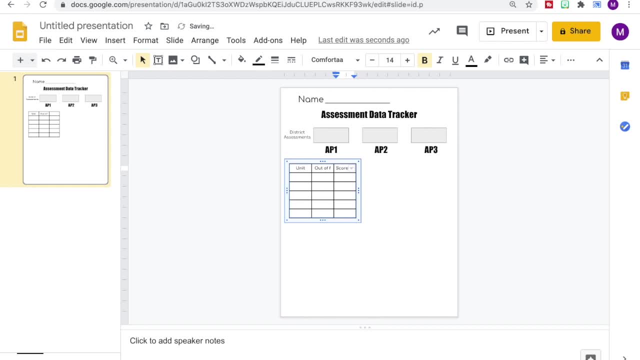 E, end, end, the preschool, the school, the classroom E, ge, E, the classroom Sанfona, a plus and E, so that is too small. I'm going to highlight all of them and then lower the font size one more time so that it fits. let's duplicate, and then I'm going to put in the unit numbers one. 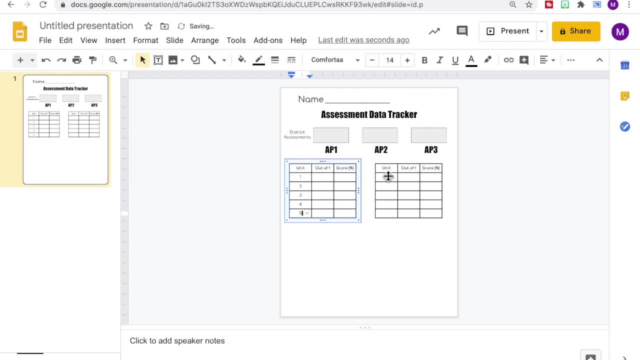 two, three. so that part is done. let's come up here and darken these boxes or these rectangles, making black, and make the border three. okay, so we're almost done. so the last thing I want to do is make a table or a chart for students to color in or shade in so that they can see the differences in their assessment. 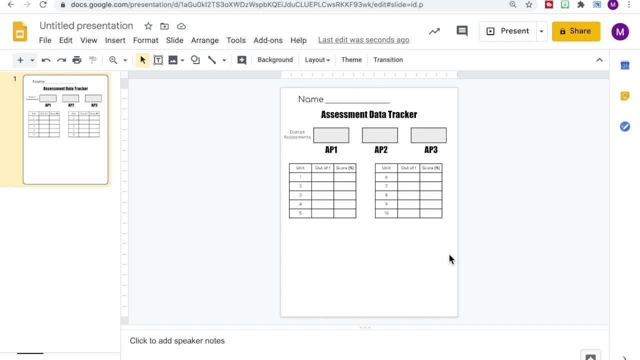 scores, so they're making progress. we want them to have a visual to represent that. so we're going to go back over to insert table. so this time I want- since there are ten units and then they can go from 0 to 100- I'm going to do a table that has 10 by 10 grid, but then I'm 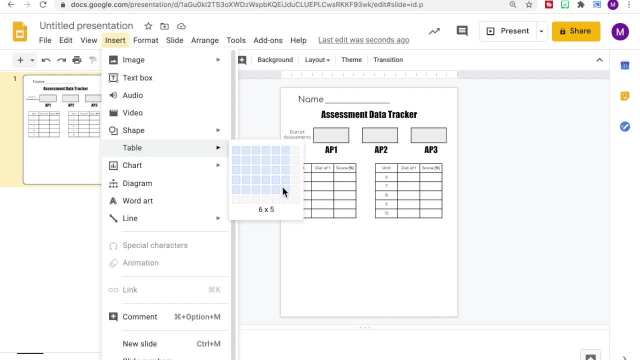 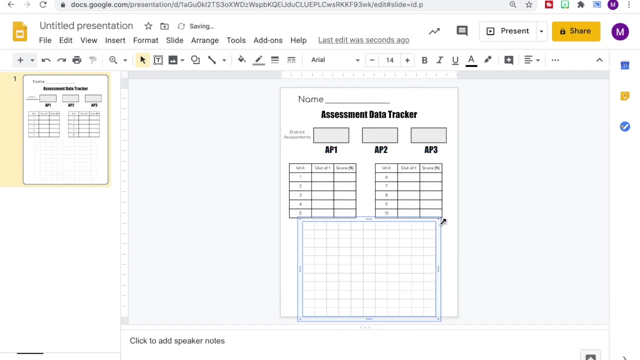 going to add in an 11th row and 11th column so that I can add my labels. so let's find 11 by 11 and then select that and then we're just gonna bring it in. let's see, that's too close. let's. 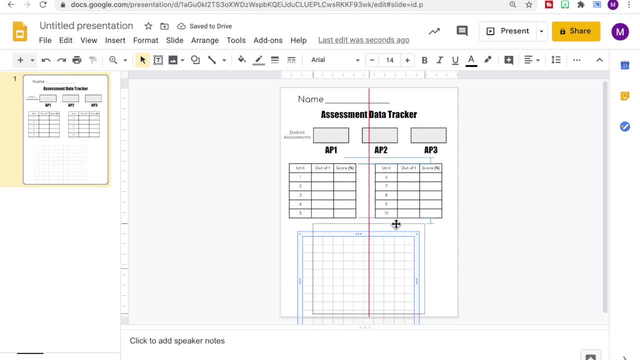 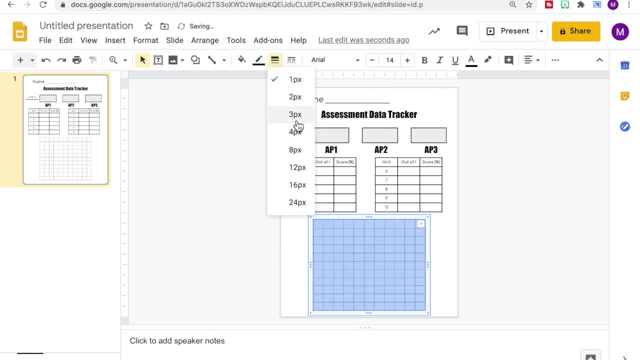 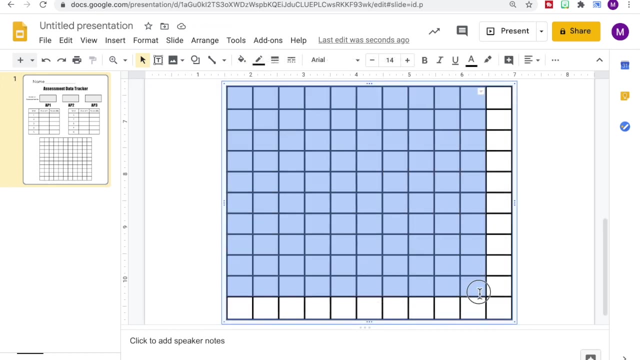 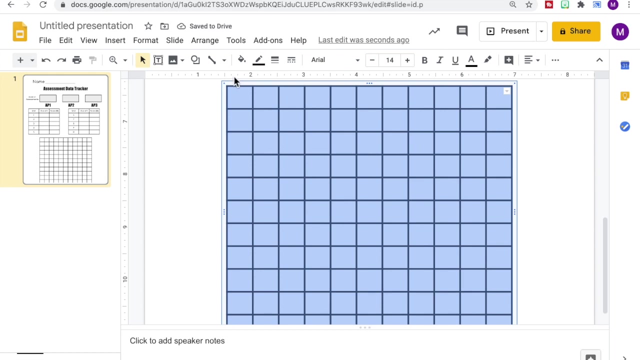 bring it down to 50. let's thicken the weight of the lines and change the color to black and the outline to three. let's highlight everything so we know that we want them all to be centered and we want that font actually. let's make the font impact. 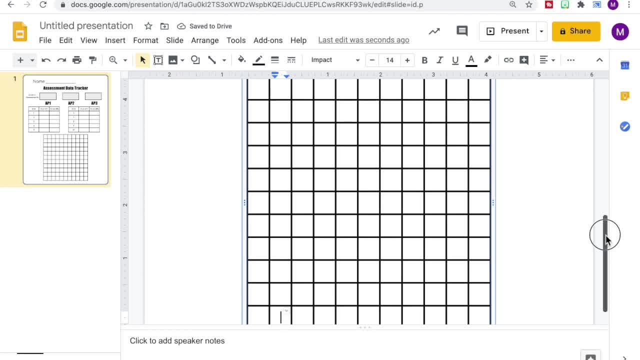 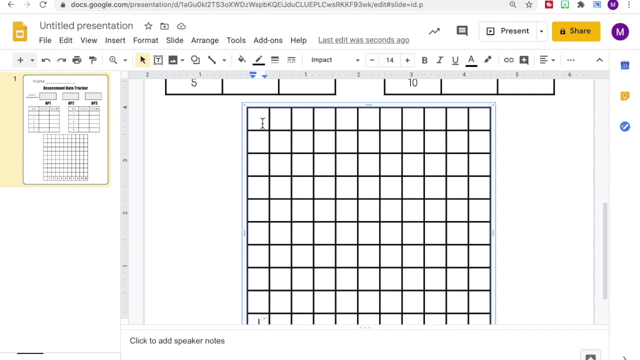 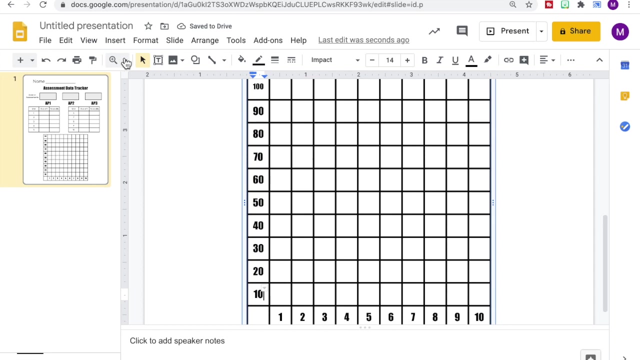 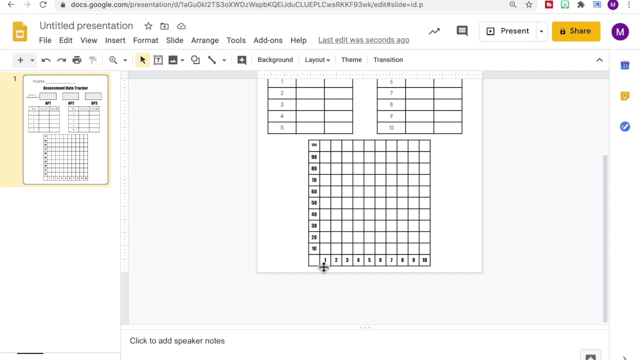 so I'm adding in our numbers on the bottom row for to represent the units. and then here are going to be the percentage. percentage is that students can earn on their assessment, so let's lower the font size for this hundred, okay. so let's zoom out slightly so we have our grid. now I want to get rid of. 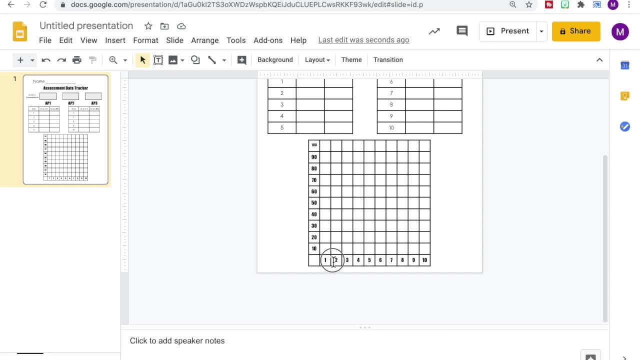 the cells around our labels. so what I'm going to do is highlight the row on the bottom- and I'm going to go over to border color and hit this transparent- and then do the same thing for the column on the left and then highlight the cells that have the missing left side. 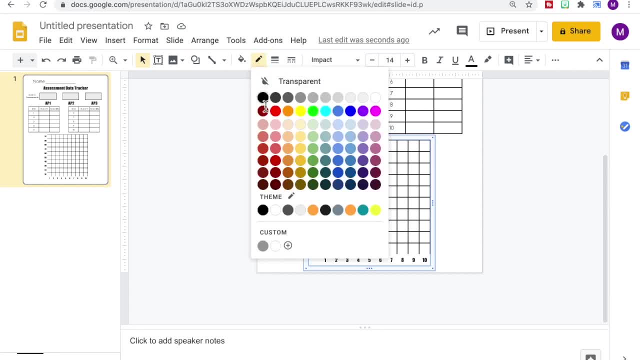 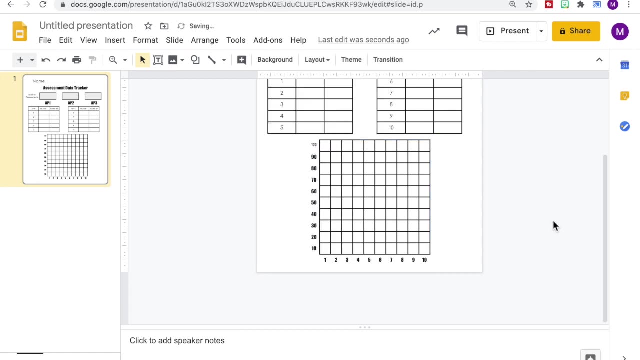 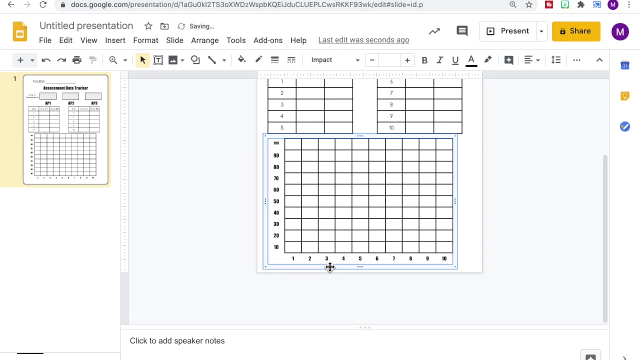 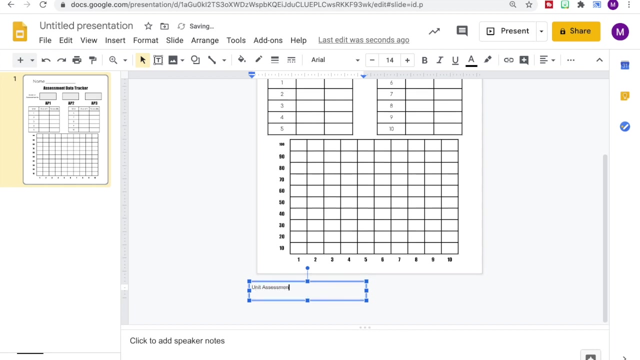 and do border color black, and then the same thing for that bottom row and there's the grid that the students can shade in. let's stretch it out a little bit, just going to add in one more text box to write that we are looking at unit assessments. that's what we're shading in at the bottom. make sure it fits. and 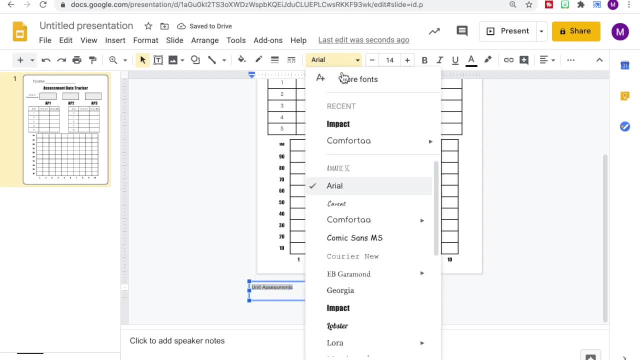 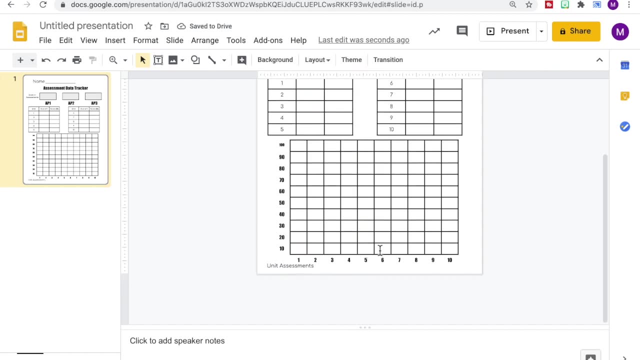 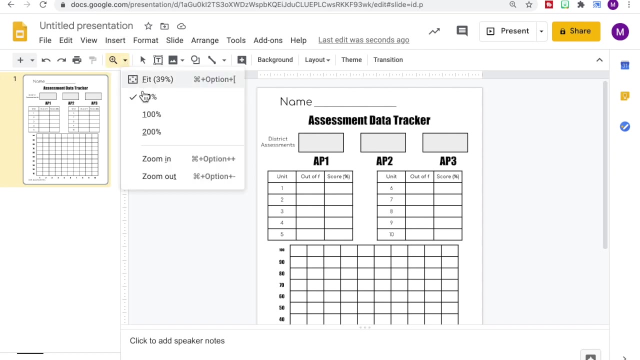 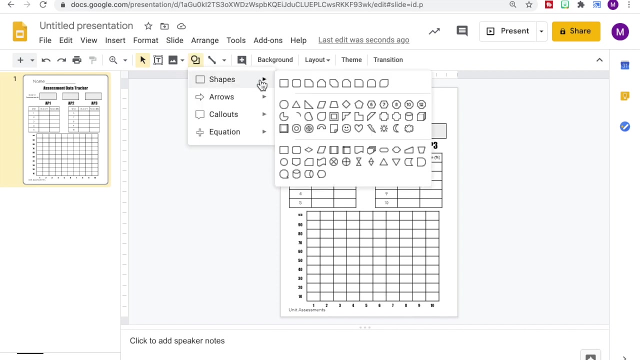 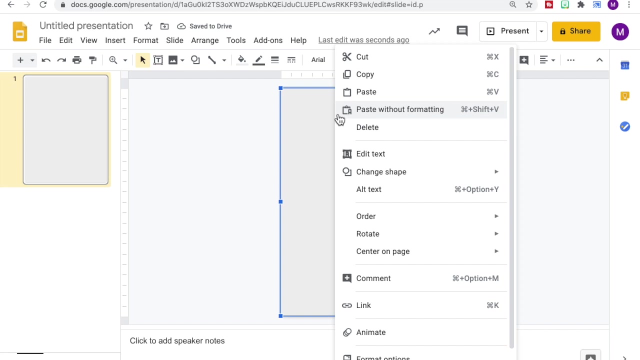 make sure it fits. let's zoom out. so the very last thing we're going to do is add in a border. so I'm going to go to shape and then click on the rectangle and highlight the entire page that gives us our shape. and I'm going to right click and then go to 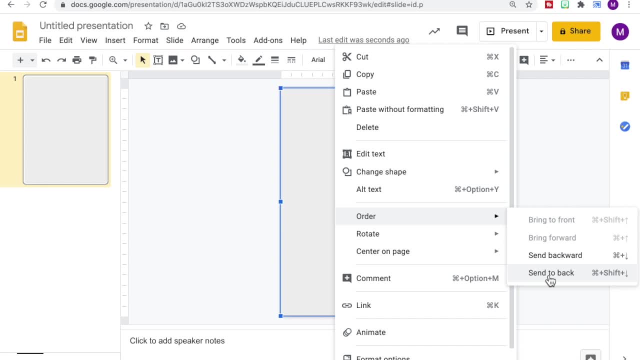 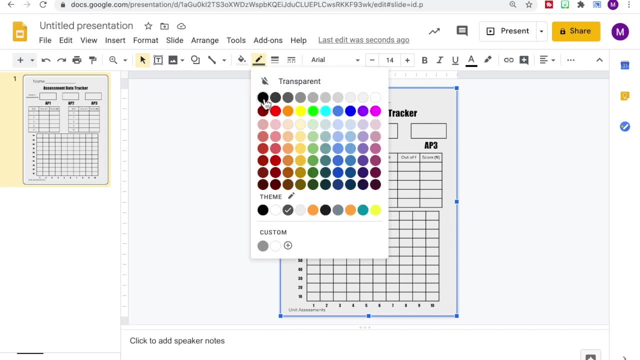 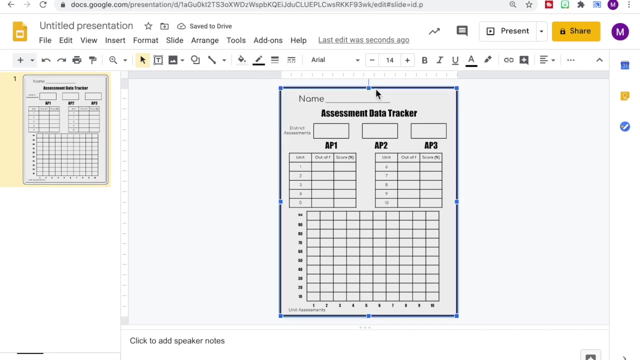 order and then go to send to image, and then go to send to image to back, and then, while the page is still highlighted, when I change the border color to black and then the weight, I'm going to change it to four. actually, let's change it to eight then we're just going to bring it in just slightly. 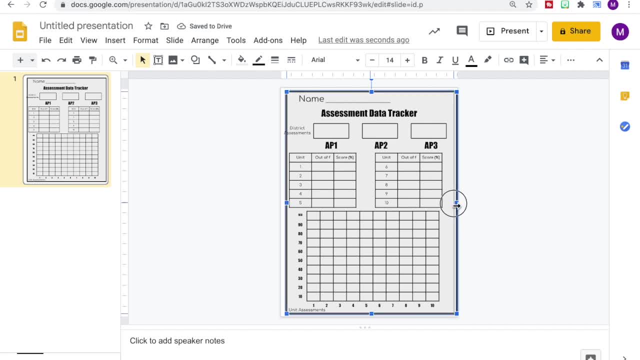 that looks good. so we're just going to bring these over. actually, I'm going to lower the font and for this one and then bring it up slightly. and there is our assessment data tracker. before we print, make sure you save it. so I'm going to type in: 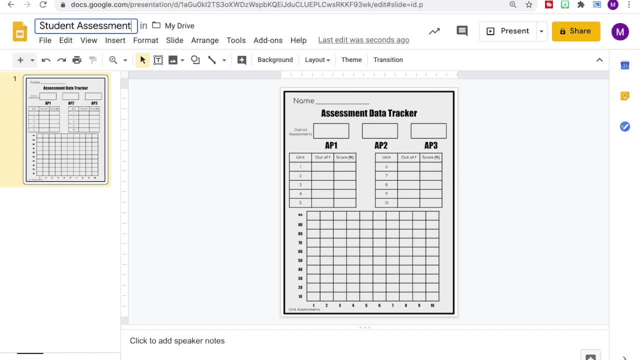 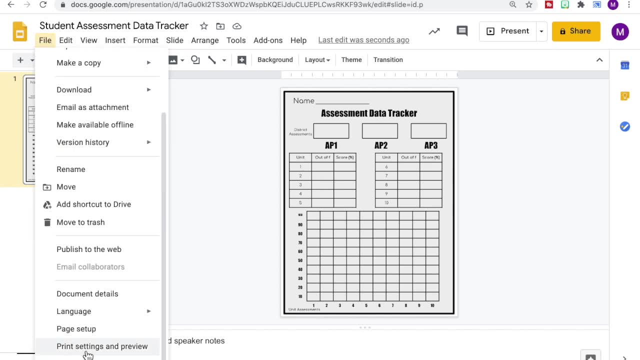 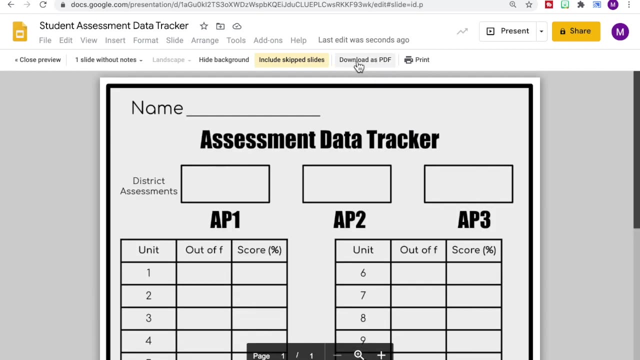 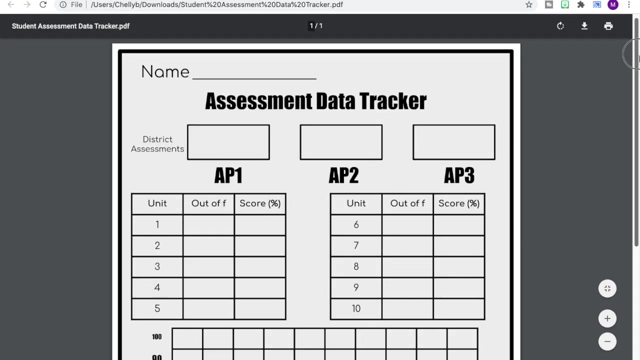 student assessment data tracker and press enter. it's saved. I'm going to go to print settings and preview and then I'm going to click on download as a PDF, and now we have our data tracker as a PDF that we can print. hope this tutorial helped you with. 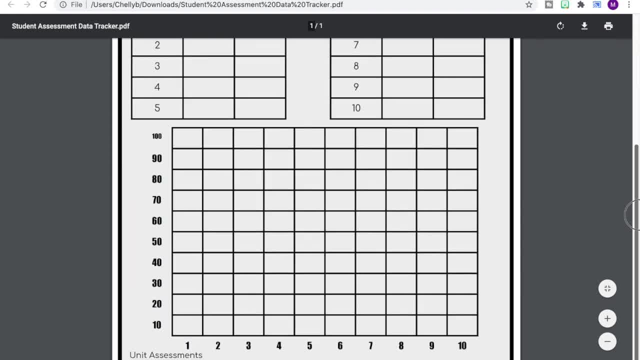 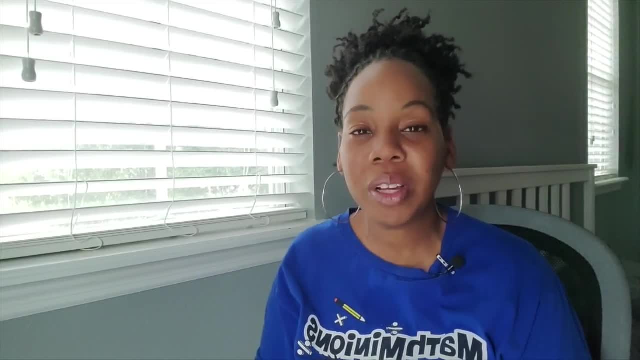 learning how to make a student data tracker. comment below and let me know what assessments you're going to be tracking with your students or your children this school year. so now day five is complete. you now have another resource that you can add to your printable math resource toolkit. and remember if you want to take 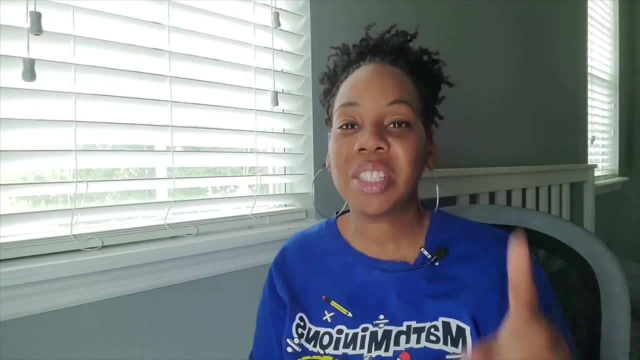 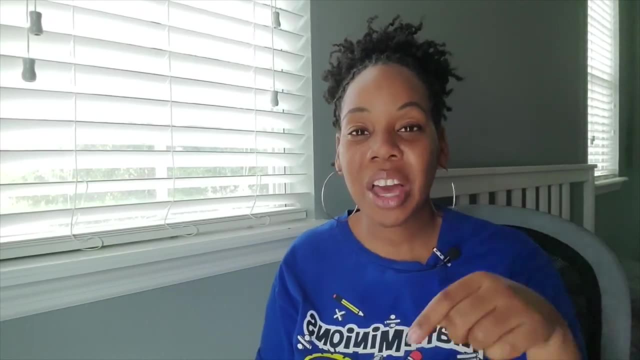 your printable and turn it into a digital resource. check out this video here and learn how to do just that, and if you want a copy of the data tracker that I showed you how to create today, check out the link in the description box below, where you can get access to today's 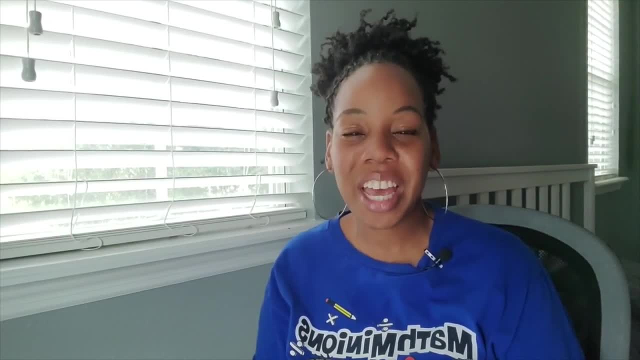 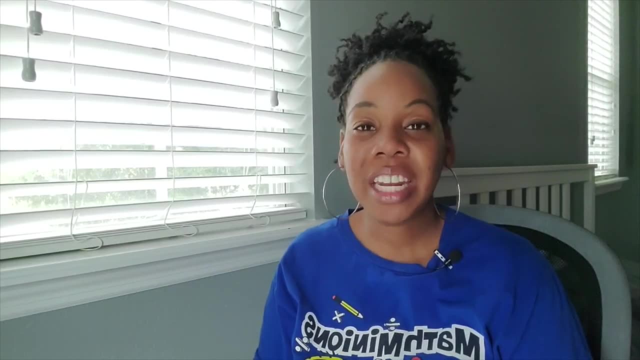 resource and all of the other resources from our 30-day challenge. if you found this video helpful, please like it by hitting that thumbs up button and consider subscribing to my channel, and if you want to be notified as soon as the next video is posted, hit that notification bell. see you in the next. video.